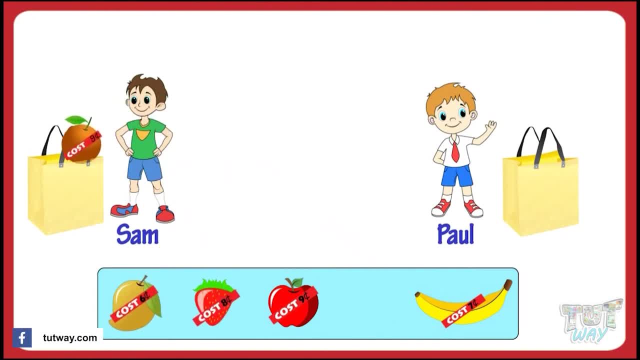 If Sam buys an orange and Paul buys a banana, who spends more? Sam spent 9 cents and Paul Paul spent 7 cents, So Sam spent more. But how many more does Sam spend? Let's find it out. Subtract the smaller amount from the bigger amount to get the difference. 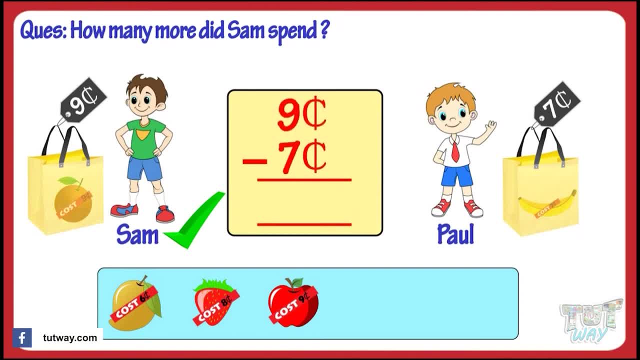 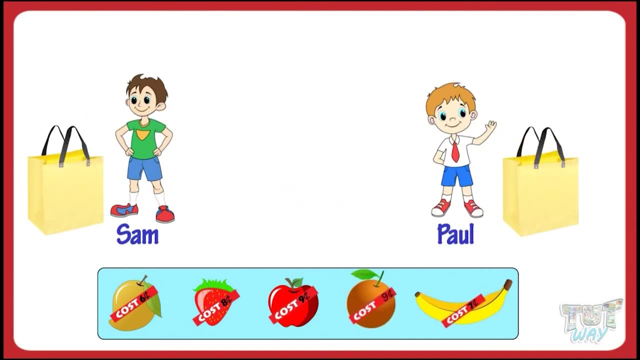 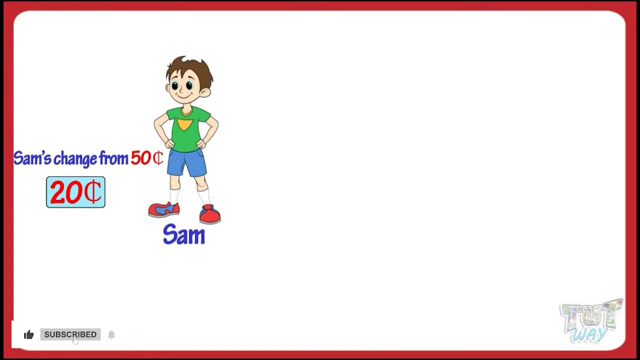 9 cents minus 7 cents, we get 2 cents. So Sam spent 2 more cents than Paul. Good, Let's take another example. Here is Sam's change with 50 cents Which of the following he did buy. Here is Sam's change with 50 cents Which of the following he did buy: 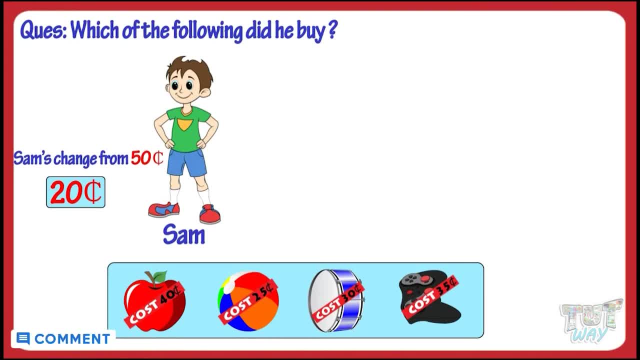 Let me help you find it out. Sam had 50 cents and his change now is 20 cents. So first calculate what he spent by subtracting the smaller amount from the bigger amount. So 50 cents minus 20 cents, we get 30 cents. 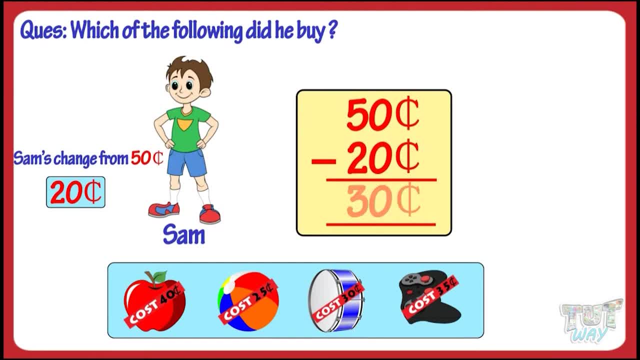 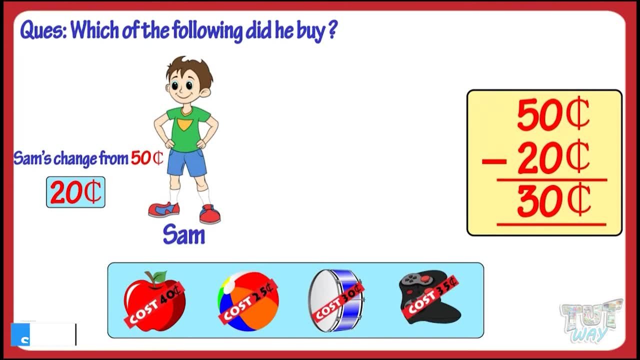 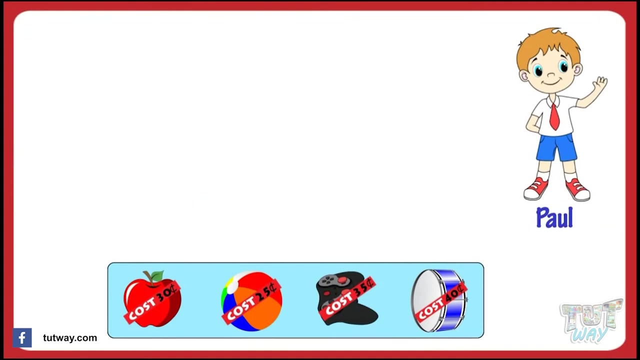 So Sam spent 30 cents. Now see which of the following thing cost 30 cents. Yeah, Toy drum cost 30 cents. So Sam bought this drum. We got it, Good Good. Now let's take another example. Paul goes shopping with 50 cents. 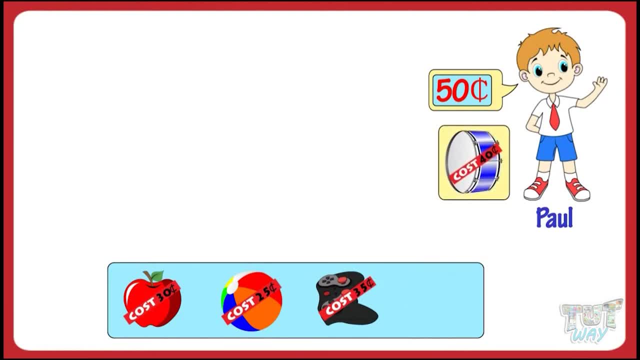 He buys a toy drum. Now calculate his change. Let me help you do that. Subtract the amount spent by Paul from the total money Paul had, So Paul's change would be 10 cents. Let's take another example. Sam goes shopping. 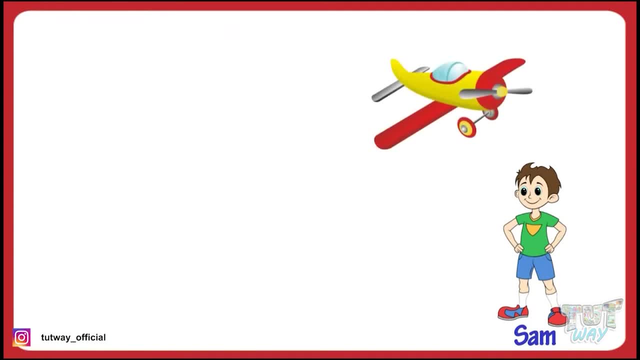 He chooses an airplane to buy for himself. Oh wow, It's on sale. That is, earlier it was for $10., But now it is for $5.. So how much money will be saved if he buys this toy? Let me help you calculate. 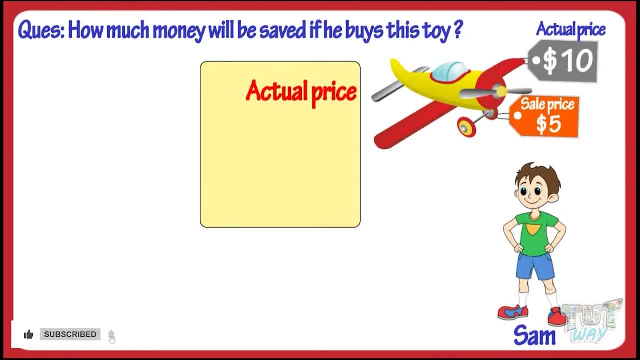 You have to find the difference between the actual price and the sale price. That is, we will be subtracting $5 from $10. To get the money he will be saving. We subtract $5 from $10. To get the money he will be saving. 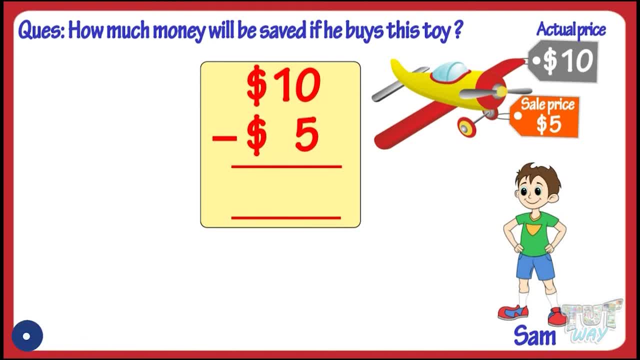 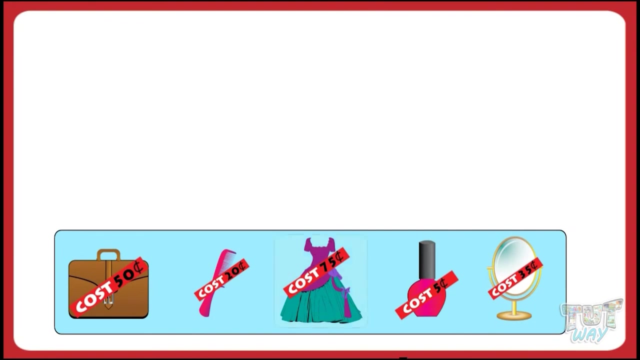 Yeah, This is a difference of $5. So $5 will be saved. Good, Let's take one more example. Here are a few things with their prices mentioned. The cost of a dress is 75 cents. The cost of a handbag is 50 cents. 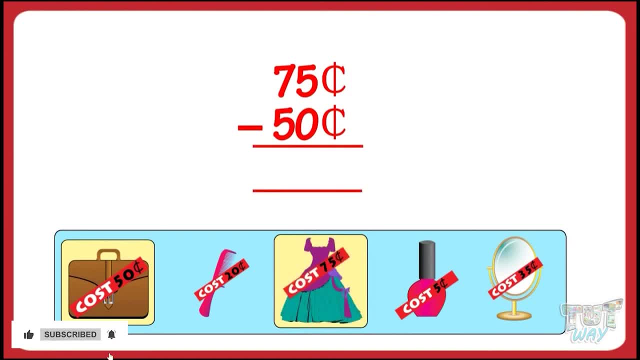 So cost of dress is more than that of a handbag. But how much more Can you calculate? Let me help you do that. You have to find the difference between cost of dress and the handbag. So subtract the smaller amount from the larger amount to get the difference. 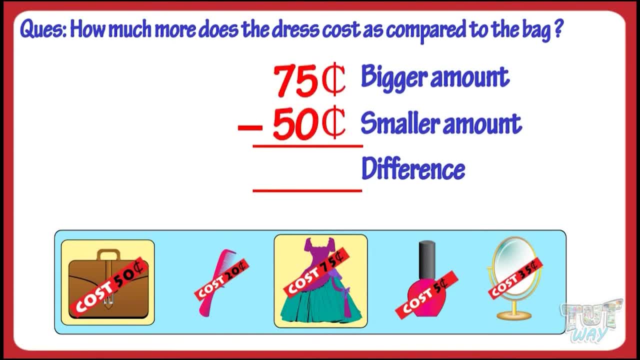 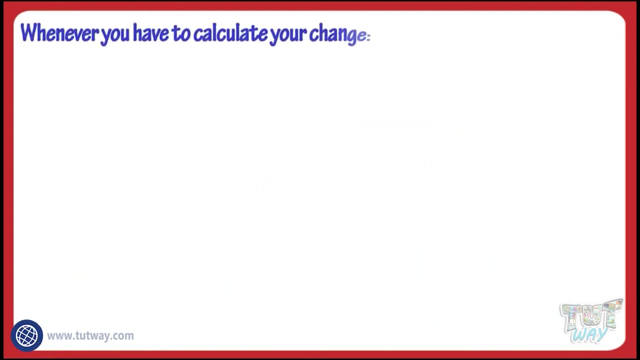 75 cents minus 50 cents, You get 25 cents. So dress costs 25 cents more than the handbag Good. So what we have learned? We have learned that Whenever you have to calculate your change, subtract the money spent from the total money you started with.